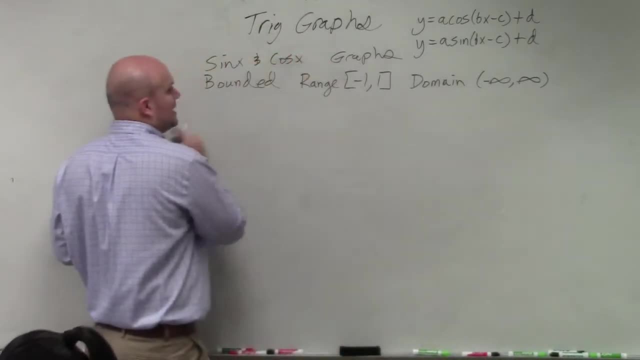 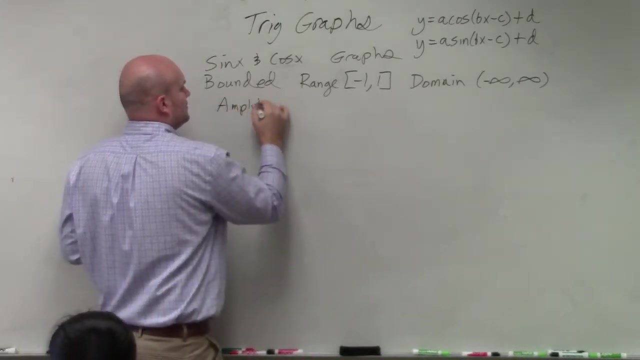 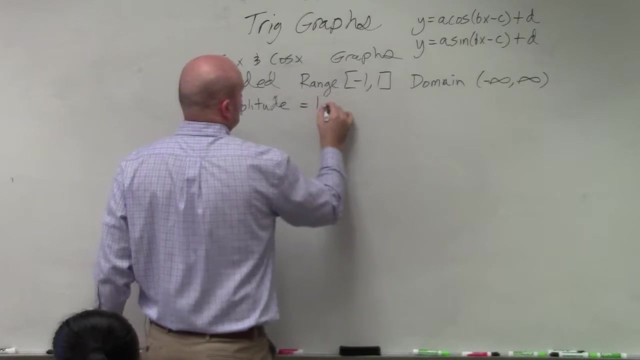 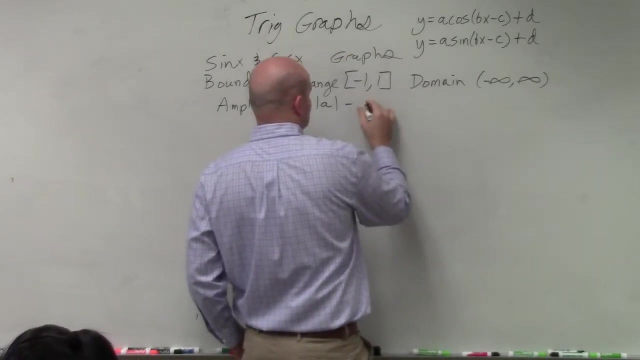 we're going to take a look at our characteristics of our graphs. So A can affect our amplitude And basically our amplitude is going to be the absolute value of A. Amplitude is going to be the absolute value of A, which is basically just means the half distance. 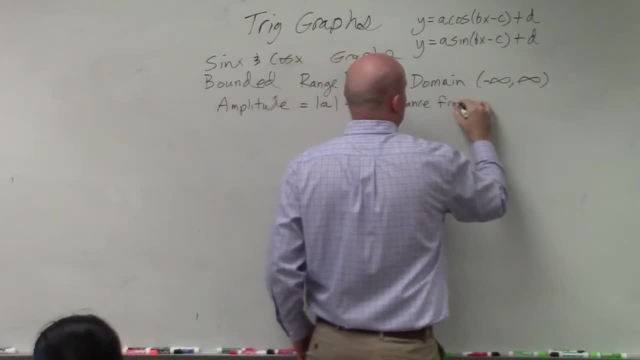 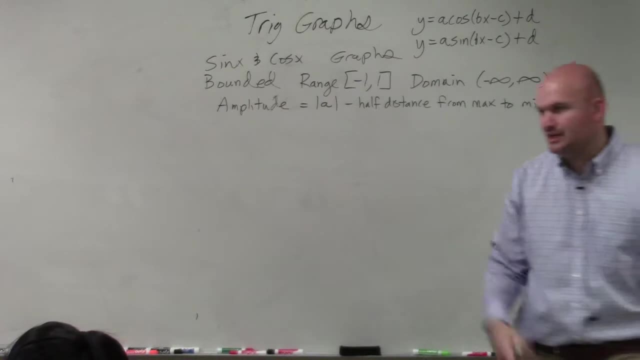 From your max point to your min. Okay, That's really what the amplitude is representing. It's the half distance. However, the amplitude is just whatever the absolute value of A is. So when you're going to be asked tonight or today, 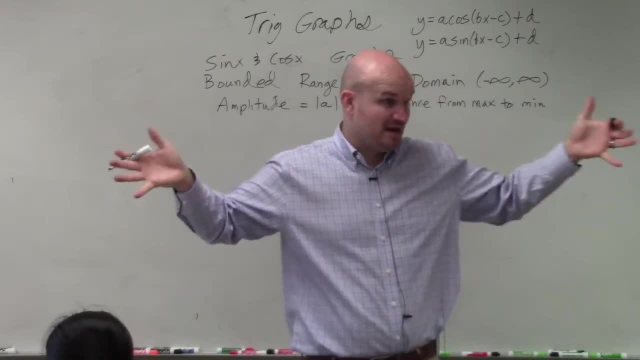 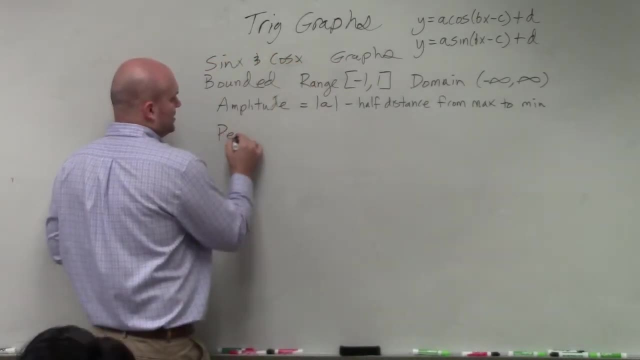 hey, what's the amplitude? Just find A, which is what is being multiplied by your function, and then identify the amplitude, Or then just take the absolute value. The next thing we're going to talk about is the amplitude. The next thing we're going to talk about is the period. 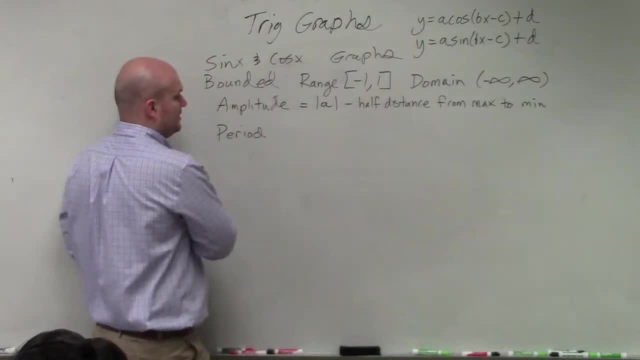 And again, this is true for sine or cosine, It does not matter. The next thing is going to be the period, And the period is simply 2 pi divided by B, And that's actually the absolute value of B. It doesn't matter if B is positive or negative. 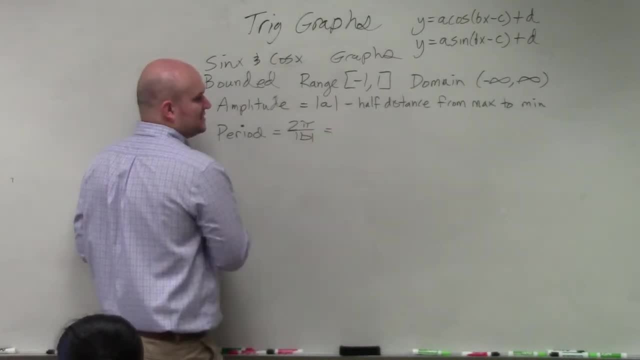 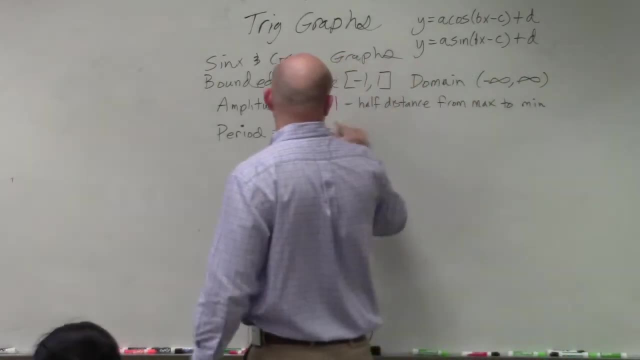 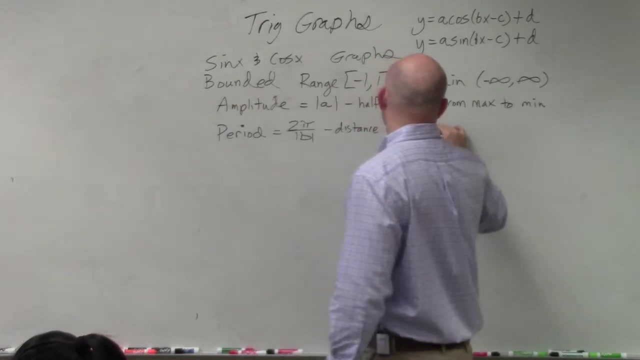 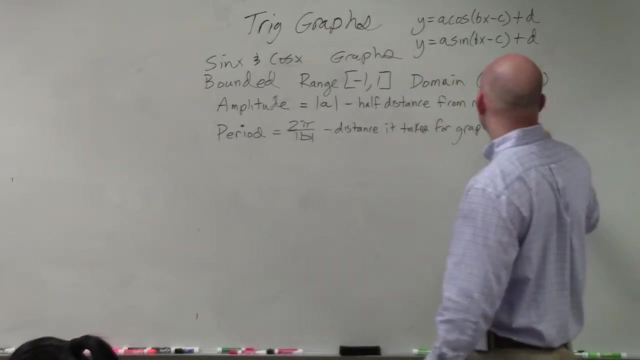 So 2 pi divided by the absolute value of P, And basically the period is basically saying how long it takes the graph to repeat itself Or to complete itself, to repeat or to complete a cycle. And if you guys look at the graph here, 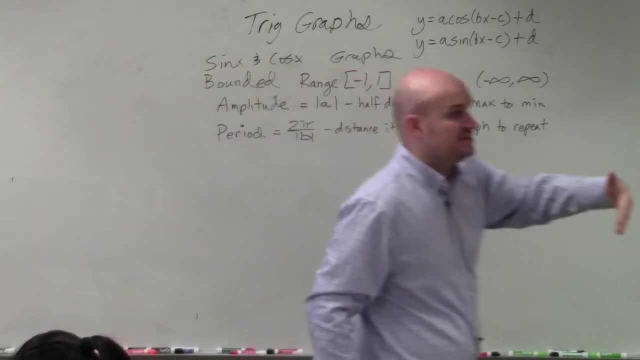 remember pi was 3.14, right, And 2 pi was, you know it would be 6.28.. Look at this, Look at the cosine graph for a second Look at the cosine graph Starts at 0.. 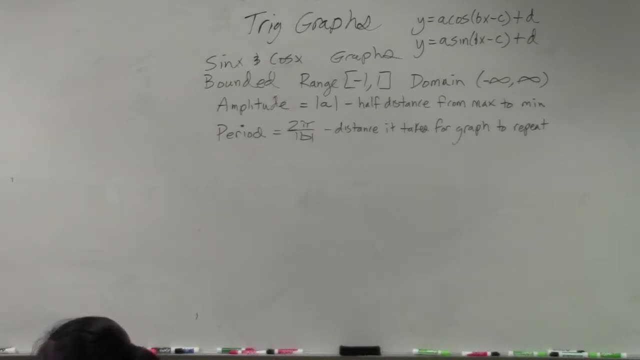 Goes all the way down And look, it doesn't. it doesn't look at where the top is. It's saying 2 pi, right, And that's because B in my general equation has 1.. So that's 2 pi over 1..